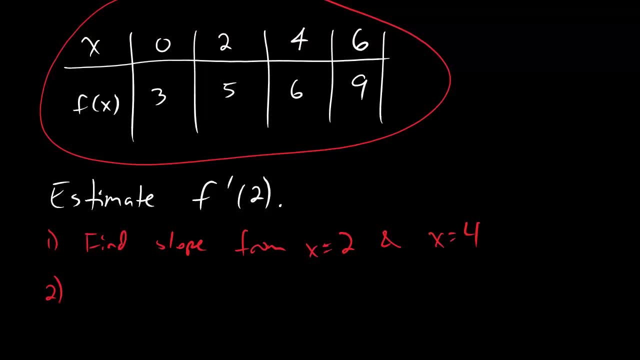 We could also start at 2 and move to the left. So that's the next thing we're going to do. We're also going to find slope from, and now let's go from x equals 0 to x equals 2.. Basically, in step 1, we move 1 to the right. In step 2, we move 1 to the left. 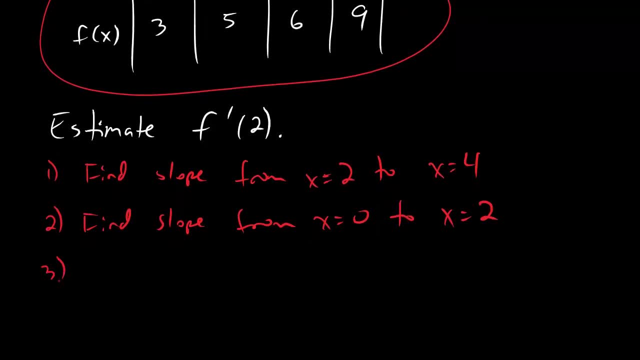 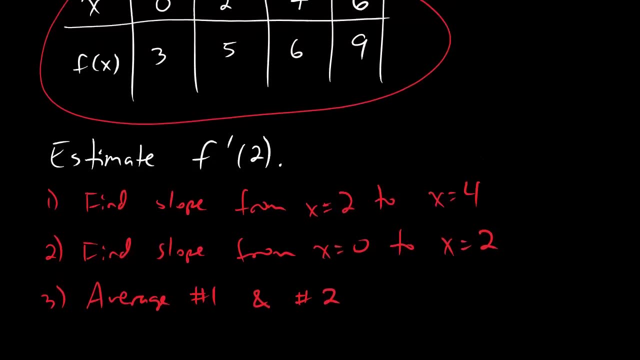 We find these slopes, and then the last thing that we're going to do is average those two numbers together, And that's exactly what you do: to estimate your derivative using a table. So let's actually go ahead and do this for f prime of 2.. 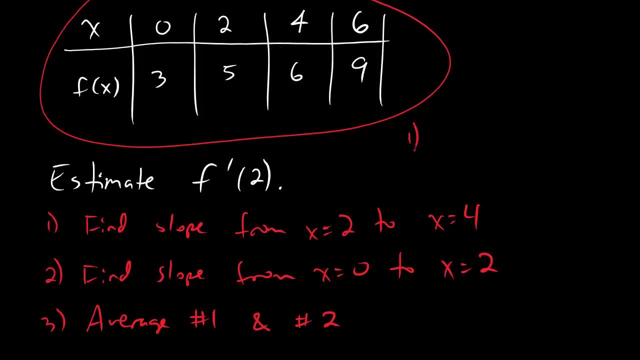 Step 1 says the slope from x equals 2 to x equals 4.. So that's going to be the change in y divided by the change in x, And that's a half. Okay, wait, so let's say this equals 1 half. 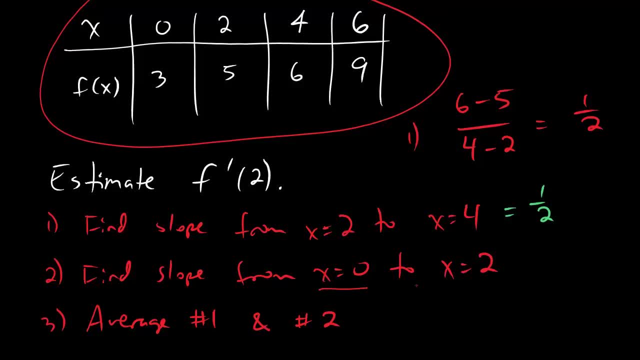 Alright, Next thing we're going to do is we're going to do the slope from x equals 2 to x equals 4.. So what we're going to do is the exact same deal, but now between 0 and 2.. Between 0 and 2, we're looking at these points here. 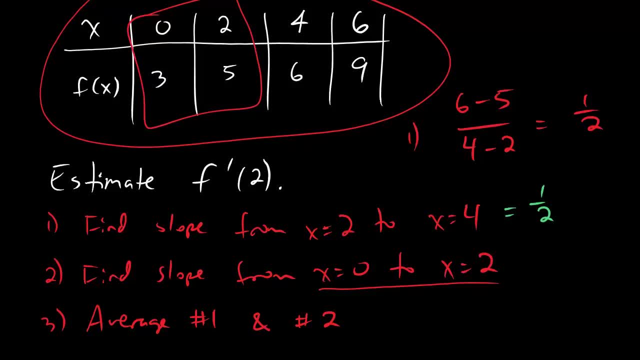 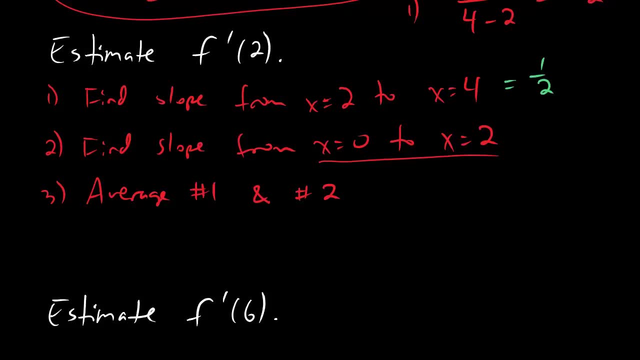 And so I need more room. Wait for it. This is going to be good, I'm going to do this thing. No, that's not what I meant. Crap, crap, crap. Wait, I'm going to do it again. 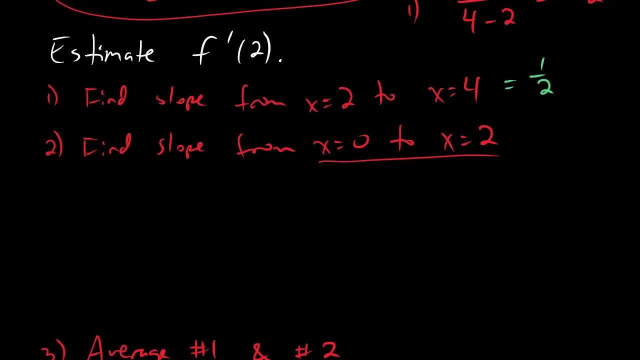 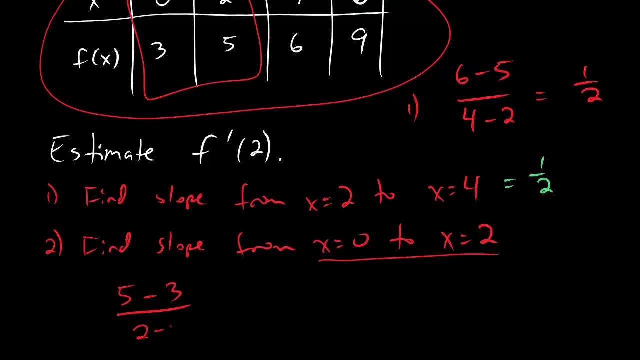 Haha, victory. Okay. so for step 2, here's what we're doing. The slope from 0 to 2 is going to look like the difference in y values Divided by the difference in x values, And from that we just get 1.. 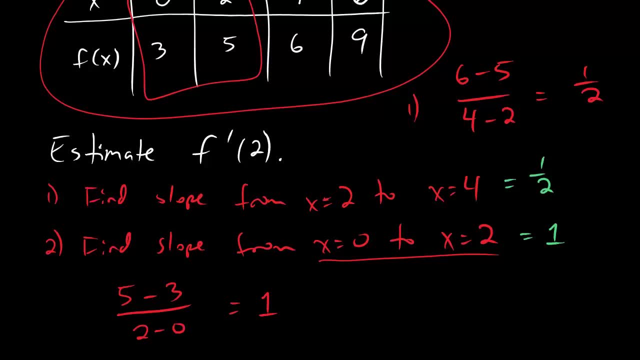 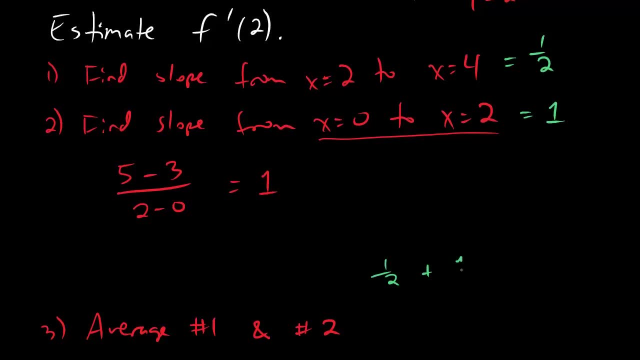 So step 1, we got a half. Step 2, we got 1.. And now for step 3, we're just going to average those two numbers together. So this is going to be 1 half plus 1 divided by 2.. 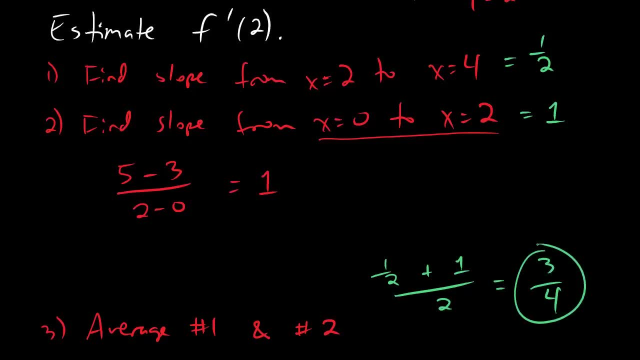 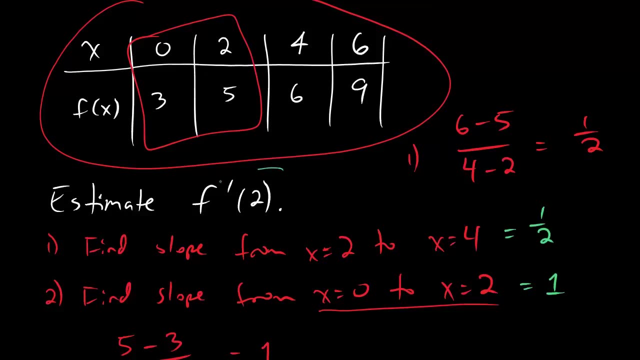 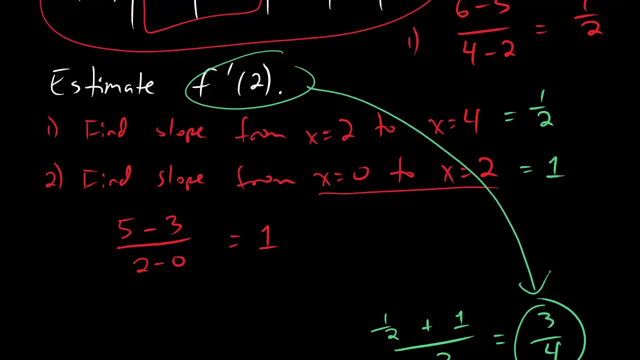 And that ends up being 3 over 4, people Bam, 3 over 4 is the best approximation you can give to the derivative Of the function with values in this table, at the point 2.. Okay, so one more time. you estimate it from the right, you estimate it from the left. 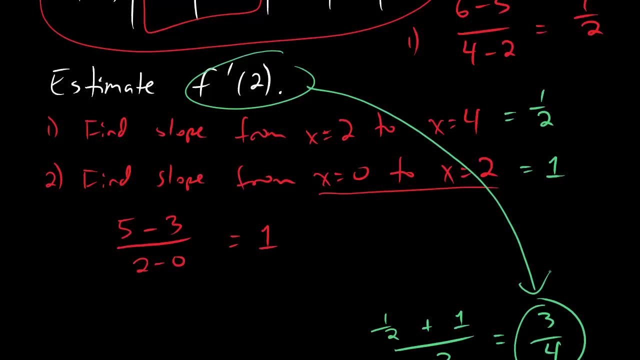 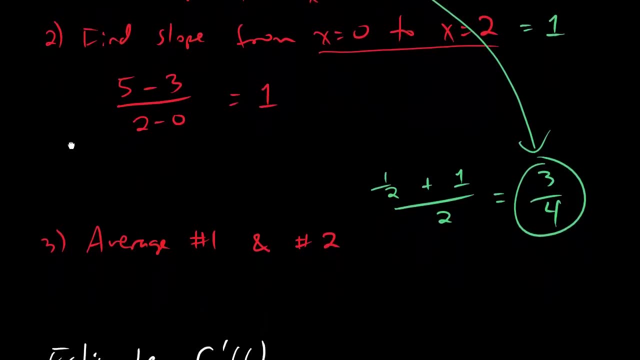 you average those puppies together. Now, if you are asked to estimate the derivative at a point where you can't always go to the right and the left, then you only stick with the one you know how to do So. for example, let's say we're asked to estimate f prime of 6.. 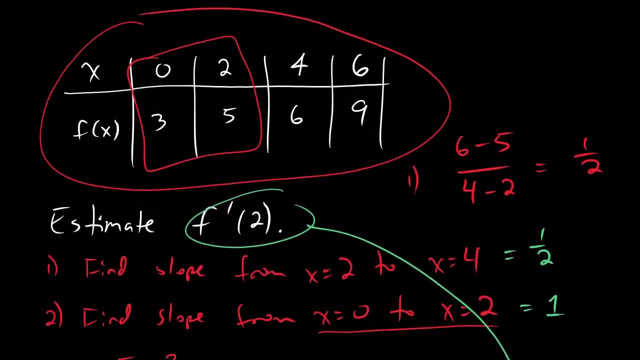 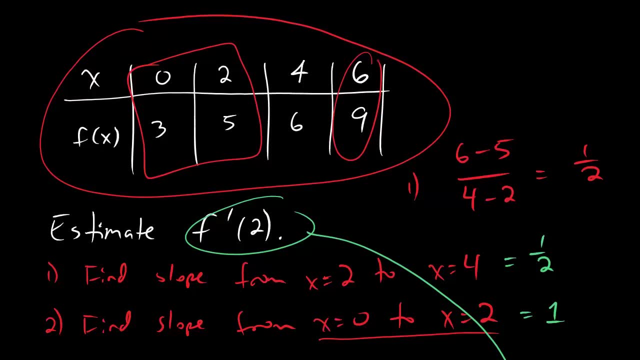 Go back up to the table. We're going to look at x prime, x value 6, and x value 6 is, of course, right. here We can move to the left, but we can't move to the right. So we can do step 2, but we cannot do step 1.. 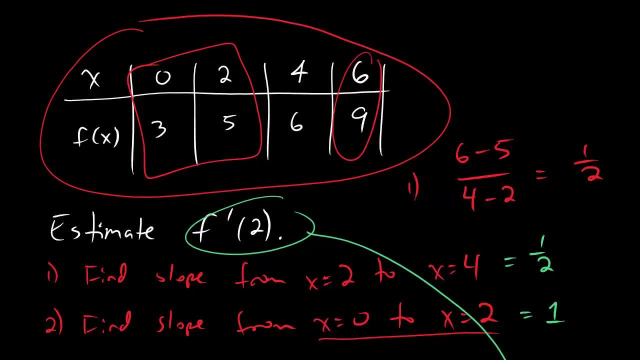 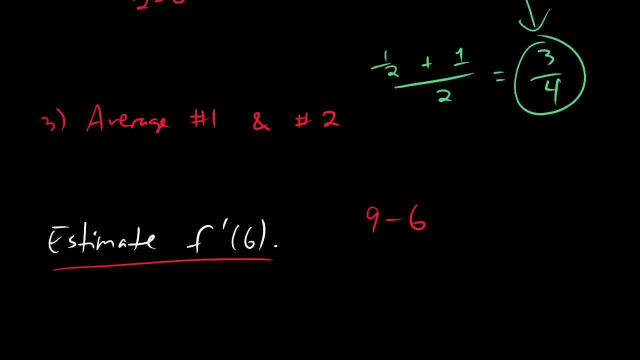 That's okay. we'll just not do step 1 in this case. So we're going to use the normal slope thing, just going from 4 to 6.. And here's what we're going to get. Change in y is 9 minus 6.. 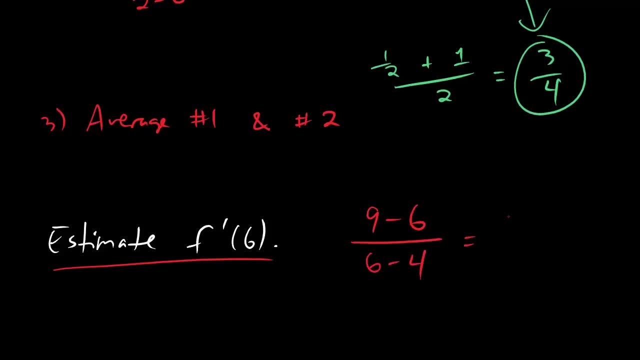 Change in x is going to be from 6 to 4. And so we get 3 halves. So if we're going from the original point to the left, we can't go one step to the right, so we just stick with that number that we have. 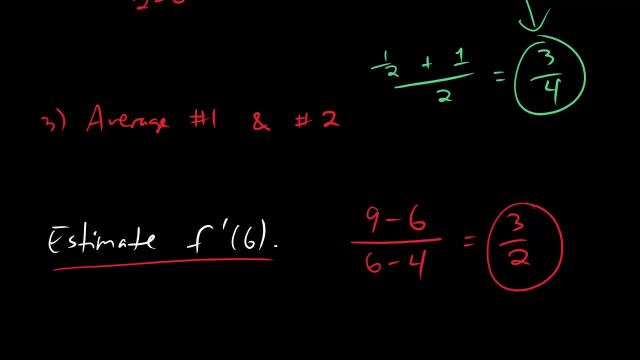 All right, dudes. that's it for estimating derivatives from a table, and I will see you in the glorious future. 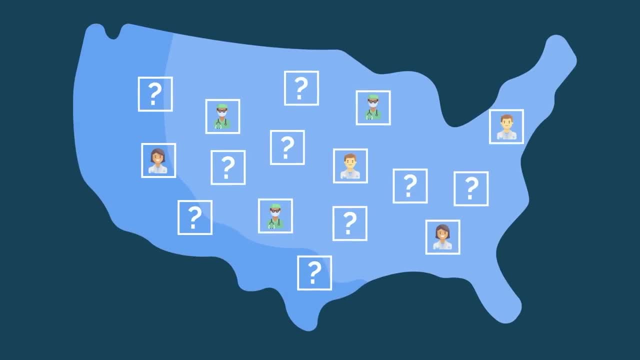 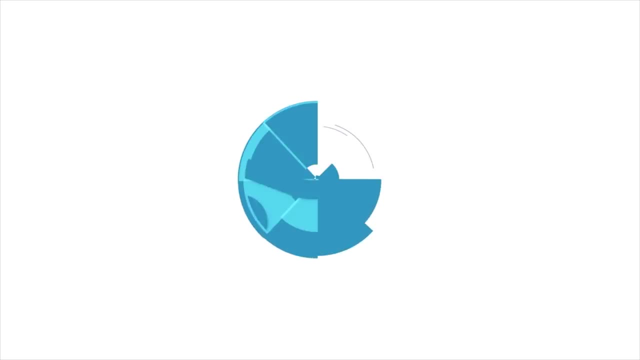 We've heard for years that America has a shortage of doctors. Sounds like an easy fix, right, We just need to train more doctors. Well, as with most things in life, it's not that simple, Dr Jubbal MedSchoolInsiderscom. According to the AAMC, we can expect shortages of between: 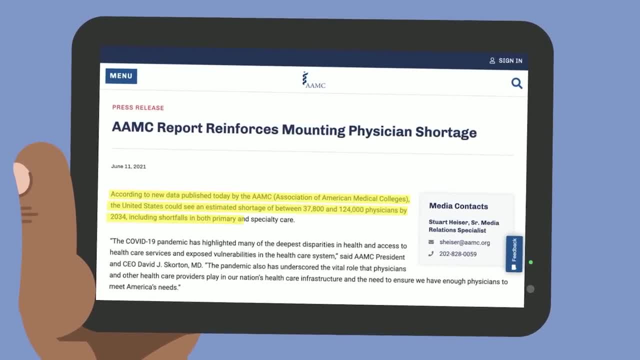 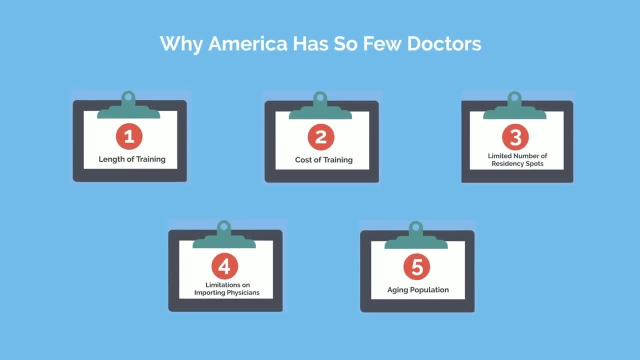 38,000 and 124,000 physicians by the year 2034.. But why is it so difficult to increase the number of physicians in the US? Here are five reasons why America has so few doctors. To start, the United States has one of the longest training pathways to becoming a physician of any.